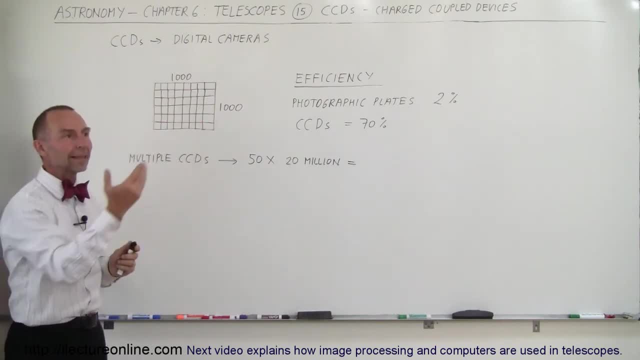 the telescope, allow it to be pointed to where you want to be looking at. then have the image fed to your computer at your desk. you look at it in real-time and you can make adjustments as you're looking at the photograph and looking at the real-time image before you make a final. 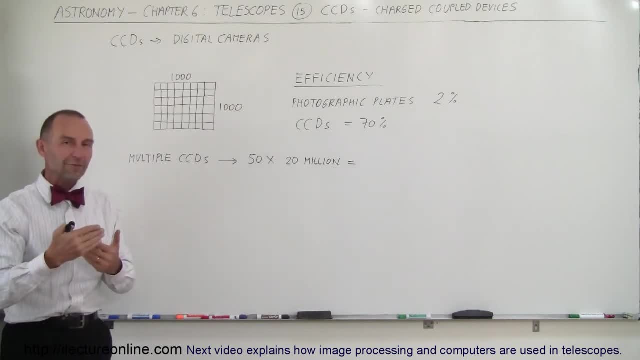 commitment to what you want to see and what you want to photograph. So we have real-time feedback, much more efficiency and we can collect light over an incredible amount of pictures. The more pixels- I should say the more pixels you have, the more accurate the 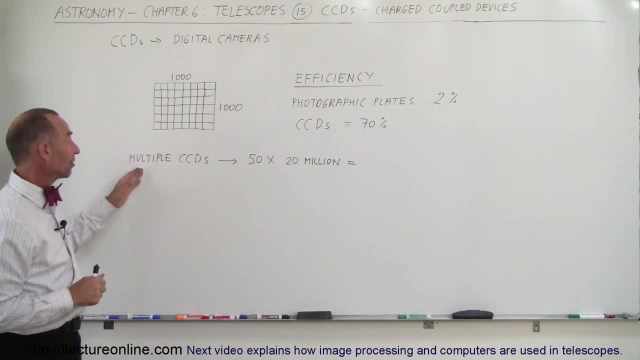 more sensitive, the higher resolution you can make your image. For example, sometimes you'll have multiple of these CCD's in the same electronic device below a telescope. so for example, let's say you have ccds that can have 20 million pickles a. 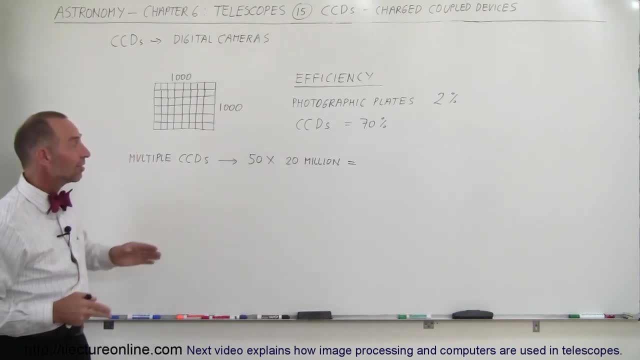 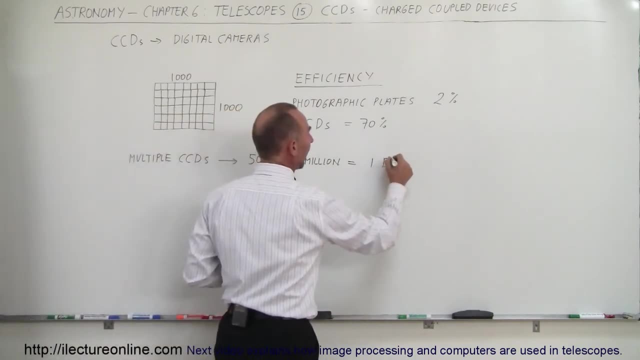 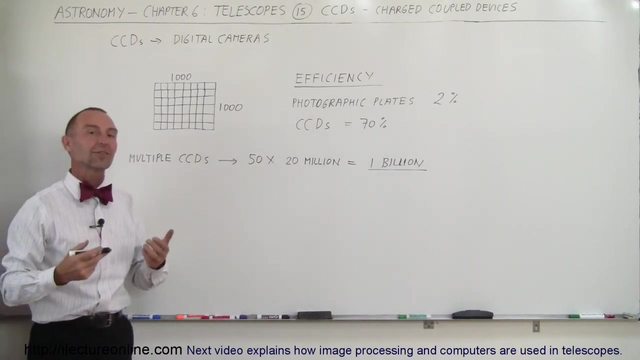 piece like four to five thousand uh ray size on each side, and let's see a fifth of them all crammed together in the same electronics. you could collect as much as one billion pixels, and in some cases we have situations where we have telescopes that will collect in excess, well, in excess of one. 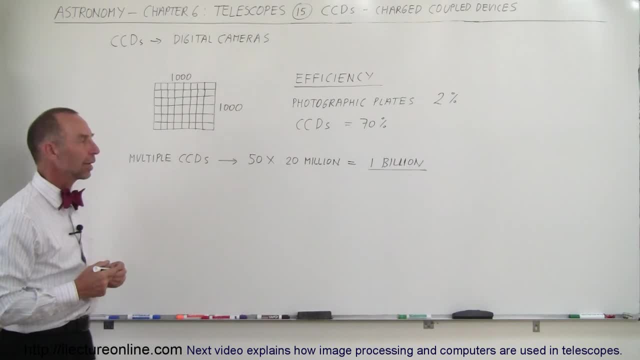 billion pixels on the photograph, along for enormous clarity, enormous detail on the photographic pictures that they take. ccds, in a very short time, have absolutely revolutionized ability for us to take pictures with telescopes. it started with very primitive types, the first ones they put up on the 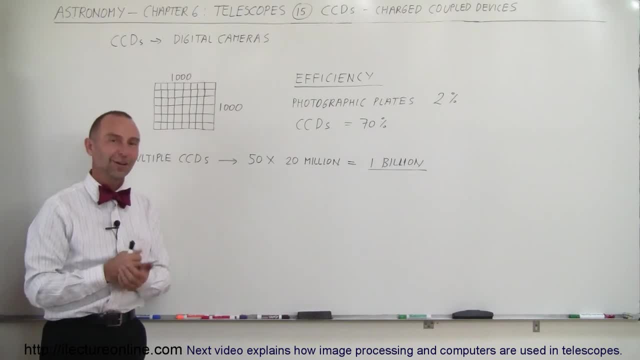 hubble were primitive compared to what we have currently in our in our modern day cell phones. we can take better pictures, in a way, with our cell phones than the hubble could, with its initial photographic plates based on the pixel. Well, they weren't really plate photographic claims, but based on the pixels that they had inside their CCDs. 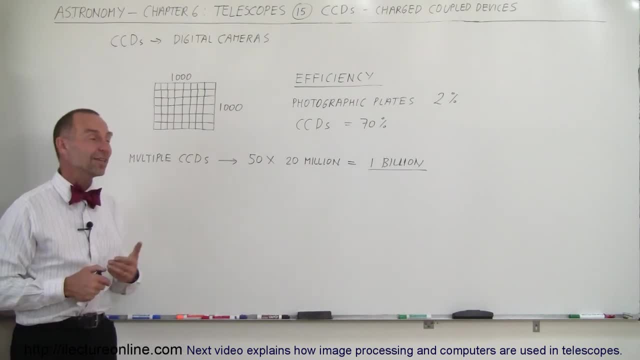 Of course, they've gone up there several times, replaced with up-to-date CCDs and up-to-date optics. Of course, they're much more powerful now than they were in the beginning, when they were put up there, But again, there's no limit as to how powerful we can make these CCDs. 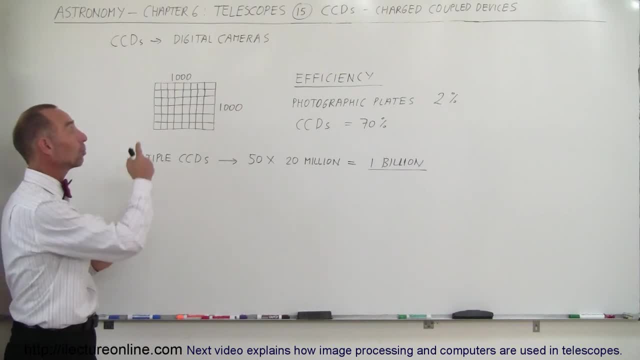 And it allows us to do one additional thing. We can actually do very nice image processing on these, which I will show you in the next video. So CCDs- something that we don't hear typically outside the astronomical world, but we call them digital cameras. 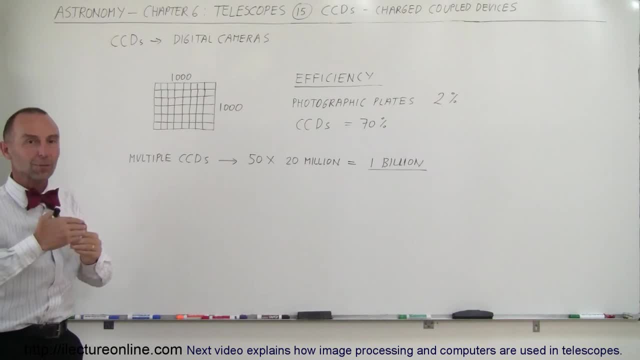 And everybody knows what a digital camera is. You can take an infinite number of pictures, store them in a computer, scroll through them as much as you want, delete them, add more to them. It's absolutely amazing what we can do with our modern technology and the modern CCDs.